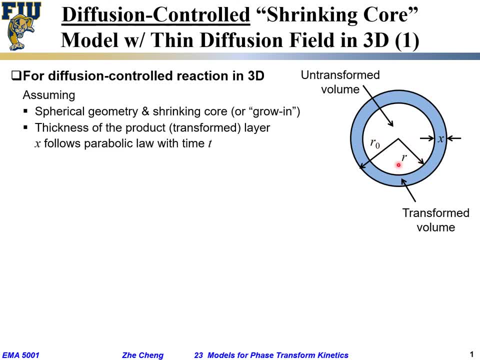 would be r0- r and the thickness for the product layer, which is the thickness for this blue shell, follows parabolic law with time. why? because we said it's diffusion controlled process. diffusion controlled process. quite often the thickness for the product follows parabolic relationship. okay, and for simplicity, let's also assume there's no change in volume for the reaction. 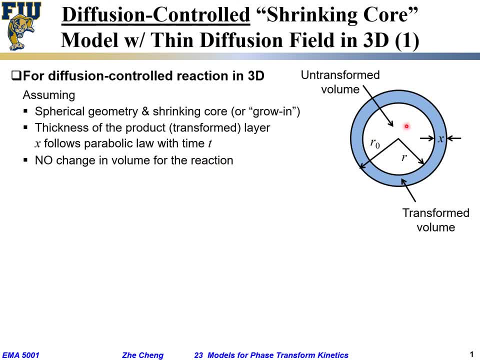 which means between the transformed volume and the untransformed volume, in the center and the transformed volume there's no volume change- net volume change during the reaction of its transformation. so with these assumptions we can build a simple model to describe the kinetics. okay, first the volume of the so-called untransformed portion, which is the sphere inside. 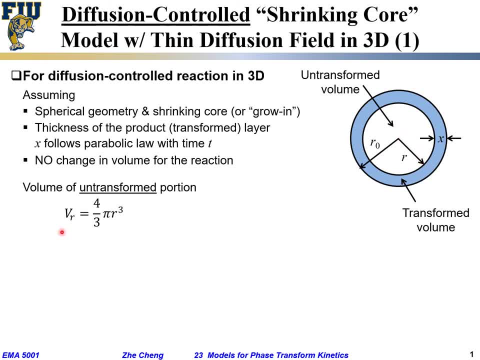 with radius of r is very simple: vr, the volume v for volume r for radius of r would be 4 over 3 pi r to the power of 3.. again, r is the radius for the untransformed volume in spherical geometry. okay, and next we are going to replace r, the radius for the untransformed form part, by r0, the radius for 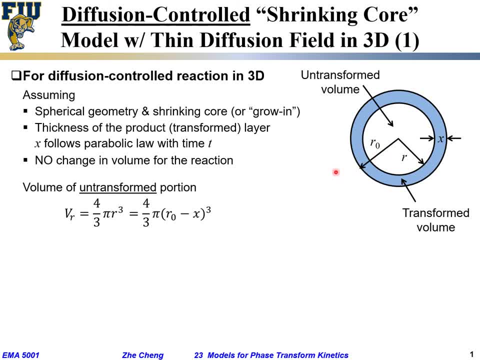 the initial sphere minus x, which is the product thickness. okay, so from here to here we just replace r with r0 minus x. x would be the thickness for the product, the shell, and which makes sense. then the fraction of transformation or the fraction of conversion, f would be given by: 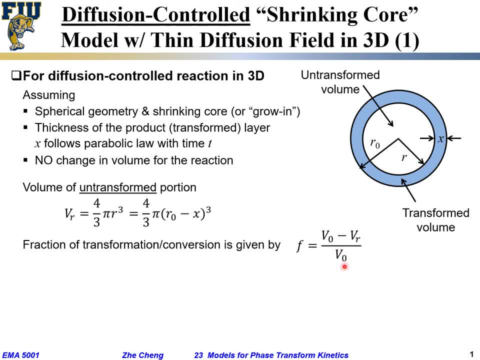 this relationship, the denominator would be the initial volume, the numerator would be the initial volume minus the vr, the untransformed volume, which is essentially the volume for this shell. okay, for this shell. so this would: this relationship ratio gives us the fraction of transformation. then consider geometrically: v zero, the initial 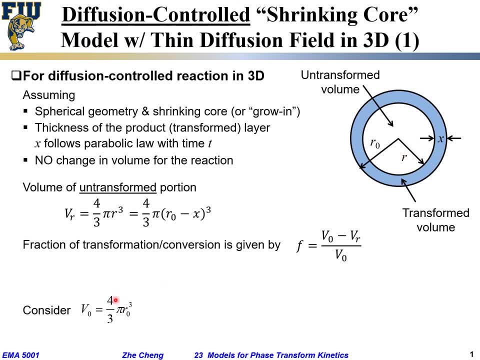 volume for sphere geometry would be four over three, pi r zero to the power of three. okay, so put this v zero and vr into this f, the fraction of conversion would be v zero, which is replaced by this sphere volume for r zero minus vr, which is given here. put it here, divided: 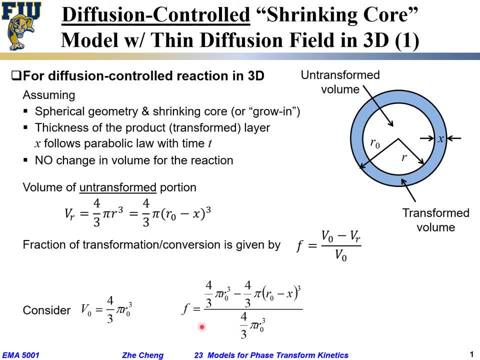 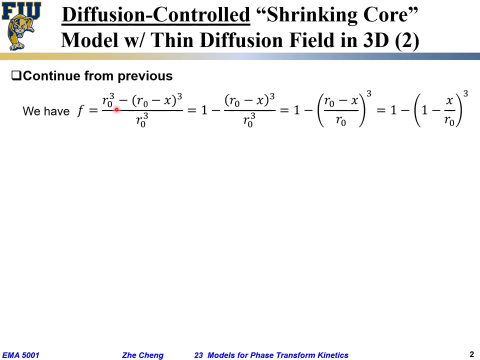 by the initial sphere volume. so this relationship gives us the fraction of transformation again very simple. the four over three pi would be cancelled from the numerator and the denominator. so this is what we have. the fraction of conversion would be r zero to the power of three minus. 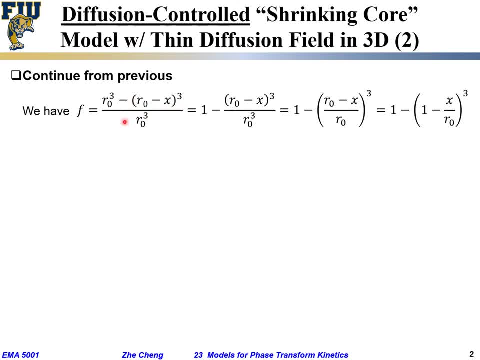 r zero minus x bracket to the power of three divided by r zero to the power of three. okay, because we get the here by cancelling the four over three pi term for each of these three terms. okay, and then we would rewrite this equation a little bit: r zero to the power three divided by r zero to the power of three, we get one minus sign. 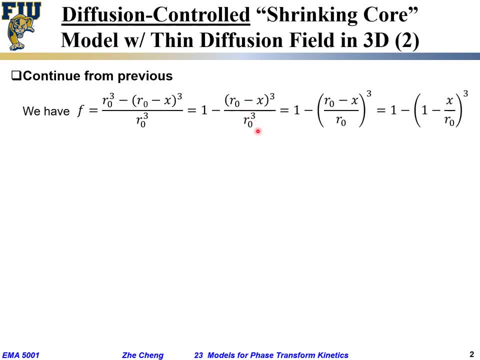 we put it here: r zero to the power of three. we keep at denominator and then the numerator would be r zero minus x to the power of three. and then we do one more transformation. we keep one minus in the front and then put the culminant power of three outside inside the 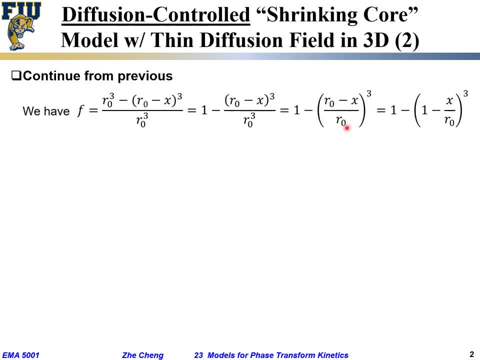 bracket would be r zero minus x, divided by Rlos x Creatused. he later defined him by the second Changes. what did we Do in the fourth equation? guess what? Dichon? Well, if we even use all of the directions which tend to break, why say and write down question mark: are allанные sign which to so? because we always take a different phrase and whenever, if we use all of the Dano from certain, And then we do a divided by road row minus X, divided by our 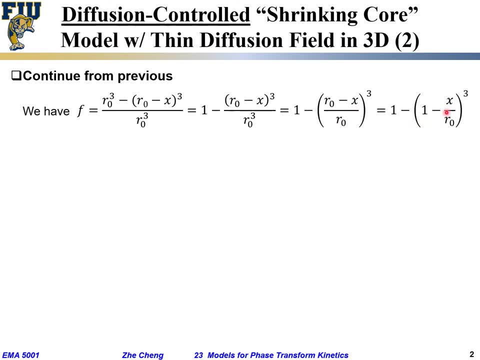 zero. all we rewrite becomes one minus x divided by our zero. okay, so this equation, give us the so called the real fraction of conversion and if we rearrange we would have: we move f to the right side, put the 1 minus x over our 0 to the power 3 to the left side and then to the power of 3. we 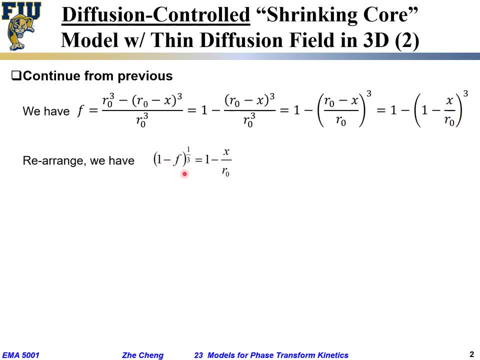 take one third of power, we would have something like this: okay, rearrange, this is what we have. and to get x, the, we are going to time our zero, we are going to move x over our zero to the left side, one minus that thing, and then times x, zero, we would get the x4 thickness for the product shell. 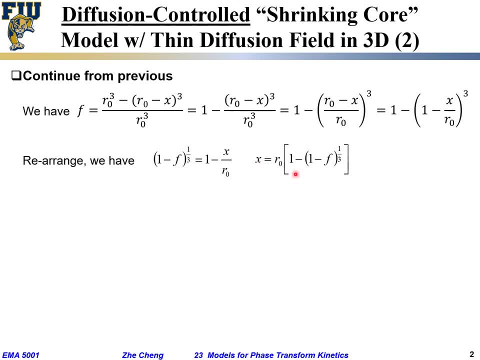 would be our zero initial radius times square bracket one minus bracket, one minus f, to the power of one third. okay, so this equation tell us that the relationship between shell thickness, initial radius and the real fraction of the combination shape- remember the thickness for the product, for this diffusion-controlled growth, satisfy. 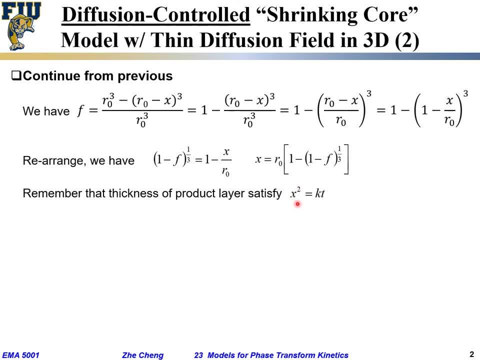 parabolic relationship, which means x square equals a constant times t. okay, if that is the case, then we will have to separate the reflected elasticurat by the function 요Н have one minus one minus f to the power three to the power of two times r zero, so essentially x. 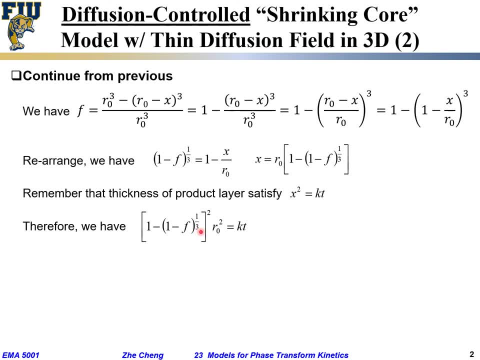 square equals kt, which is r zero square times this one equals kt. and then we can do one further manipulation: move the r 0 square to the right side. we would have 1 minus bracket, 1 minus f to the power of 3. the overall square term equals k over r, zero squared times t. okay, so now we have. 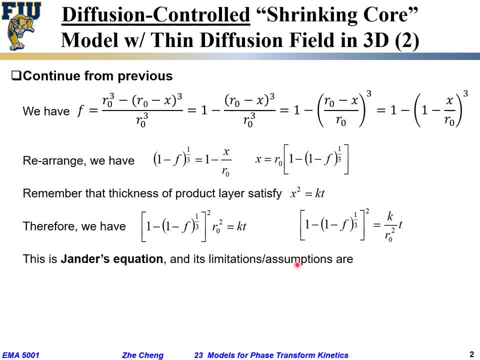 a k? t relationship which is quite often in kinetics. this is so-called agenda's equation. and next we will take the p-thanzaд. this is the k, always the k-thanza, theinas equation. and next we will take the p-theGUA and we will conclude that, if we can imagine that r néf as such,